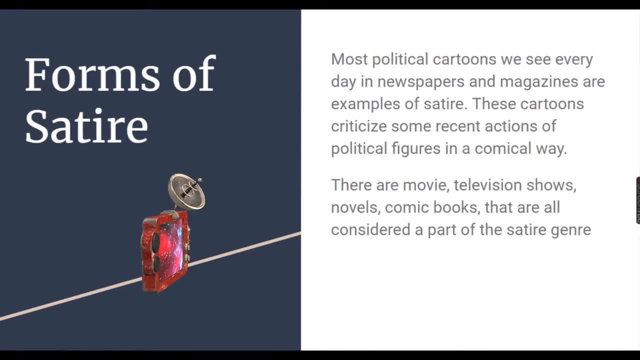 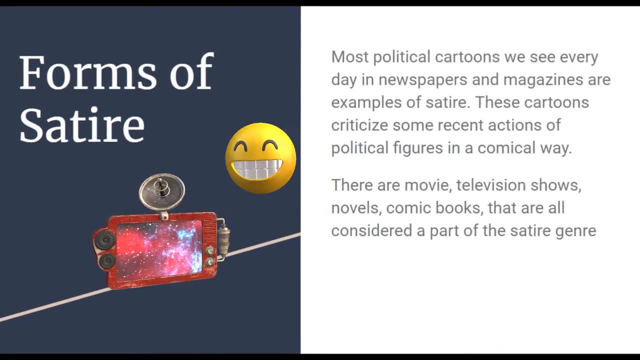 These cartoons criticize some recent action of political figures in a comedic way. Since the explosion of social media, we definitely see a lot of these political cartoons in what we call memes today. So often a meme is funny, but it's funny because it's making people laugh. 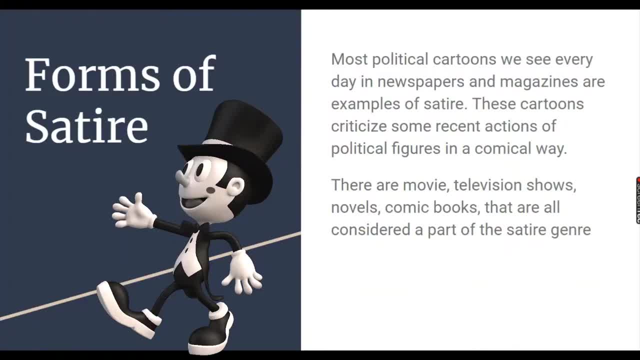 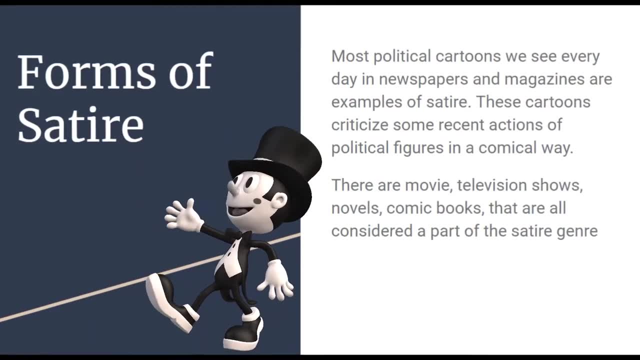 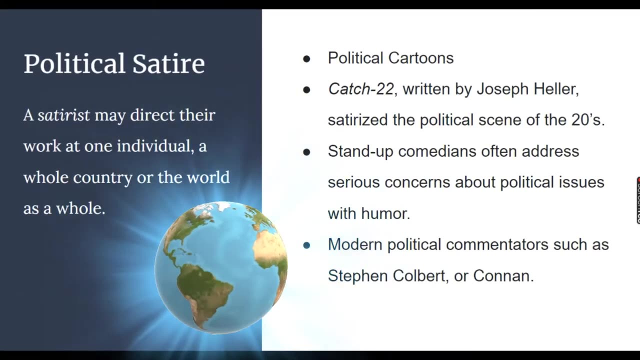 It's making some sort of statement about the image that you see in the meme. There are movie, television shows, novels, comic books and all types of things that you see today. that would be considered satire. The first thing we're going to talk about is political satire. 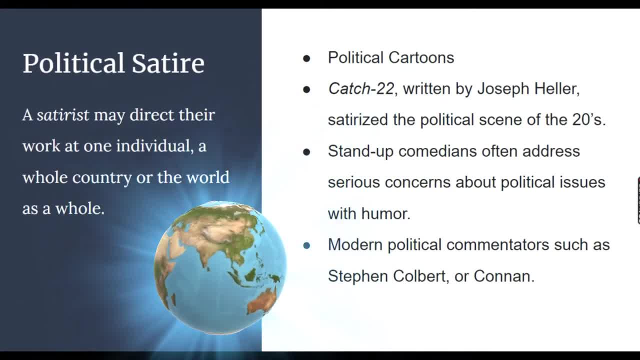 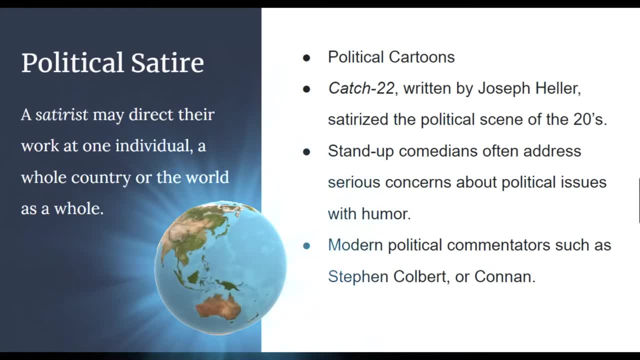 So a satirist, someone who writes satire, may direct their work at one individual. they could direct it at the whole country or they can direct it at the world as a whole. When we talk about the world, we're talking about all of humanity. 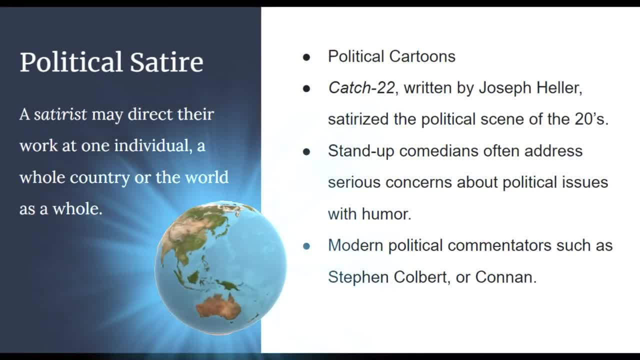 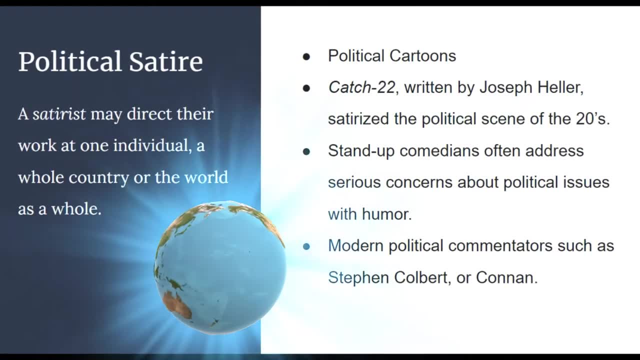 So things that are political satires would be the political cartoons or memes that you see in social media. The book Catch-22,, which was written by Joseph Heller, is definitely a satirized novel, all about political issues in the 20s. 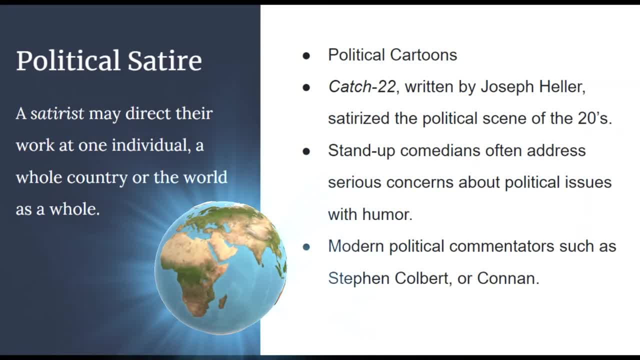 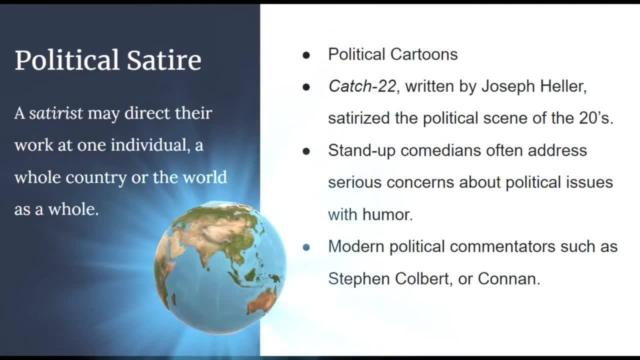 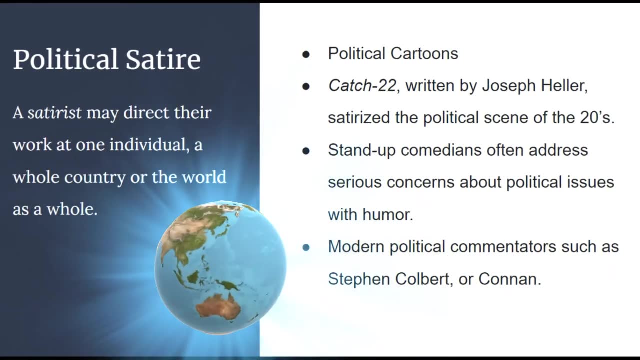 You have stand-up comedians who often talk about things going on in the world around them. All of the jokes that they would be making in their stand-up sets would be satirical. And you also have modern political commenters such as Stephen Colbert or Conan in all of those late night shows where they are criticizing the politics of that time. 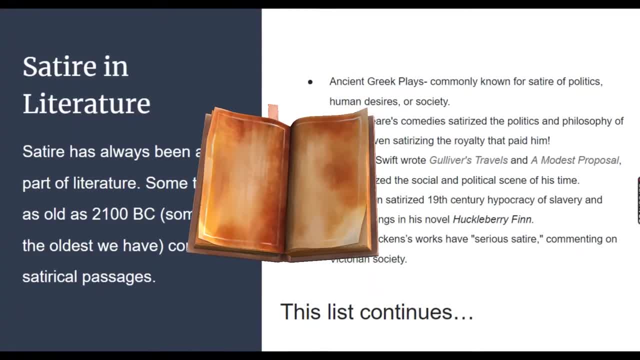 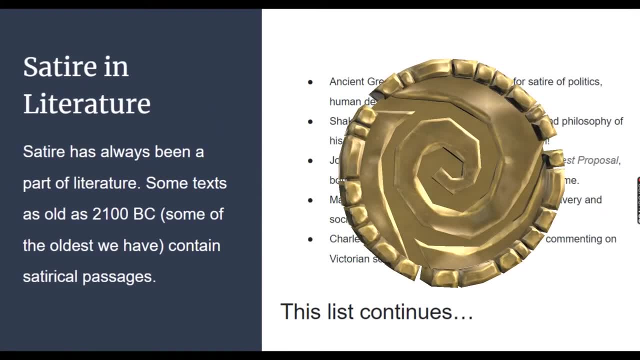 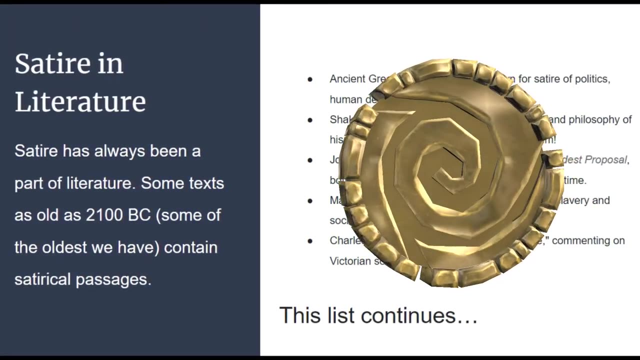 You also see satire in literature. We have seen satirical elements in literature since literature became a thing. We can find it all the way back to 2100. In some of Siddhartha or other ancient works. Some examples of this is ancient Greek plays. 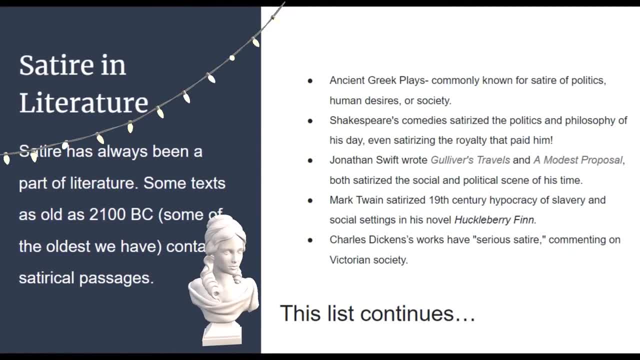 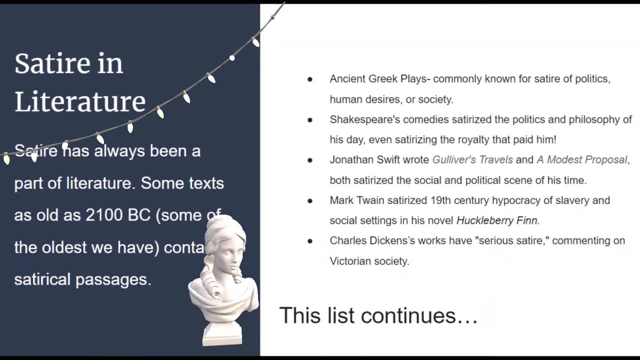 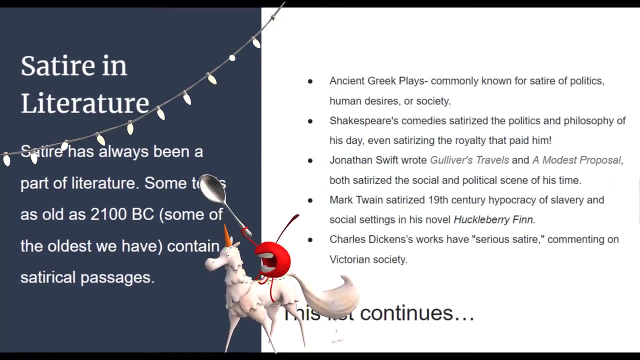 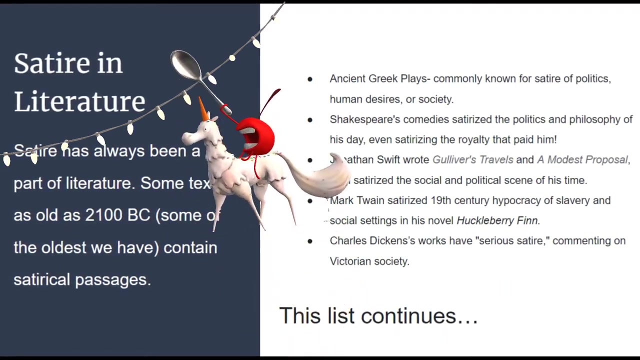 Most Greek plays that were created were going to be satirical or commenting satirically about the politics, human desires and society at that time. Shakespeare used a lot of satire in his comedies, Where he was satirizing politics, philosophy of that time period and even the royalty which were the people that paid him to work. 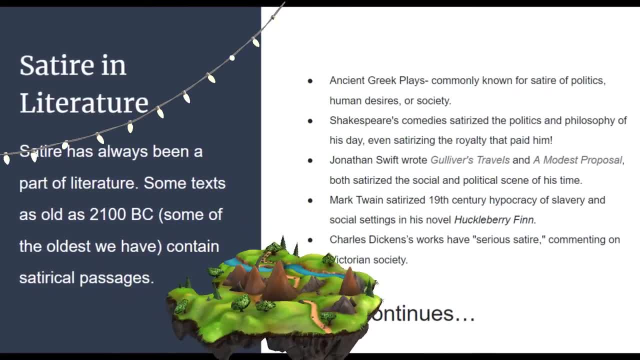 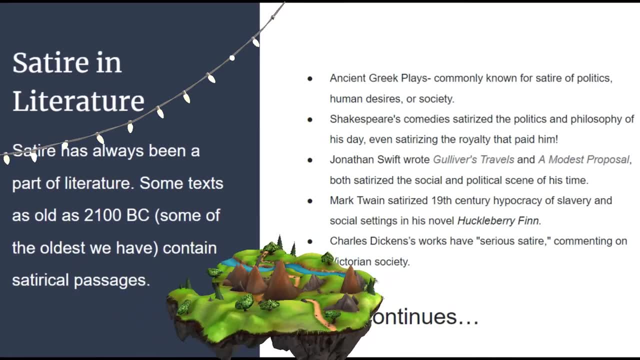 Jonathan Swift is the author who wrote Gulliver's Travels and A Modest Proposal. Both of these novels satirize the social and political sense of his time. Mark Twain also satirized 19th century Americana through his novels. 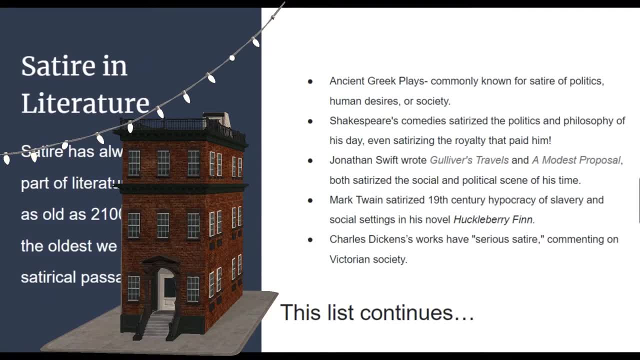 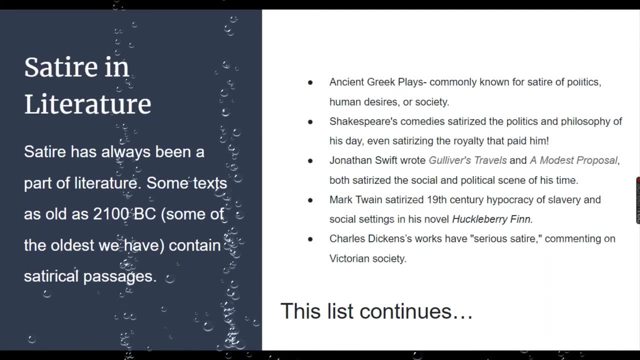 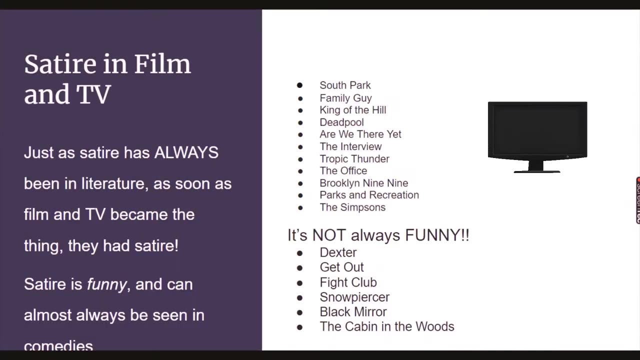 Huckleberry Finn and other works. Charles Dickens also satirized Victorian society in most of his novels, And obviously the list continues because, again, literature and satire have been hand in hand since people started putting pen to paper. We also see a lot of satire in film and TV. 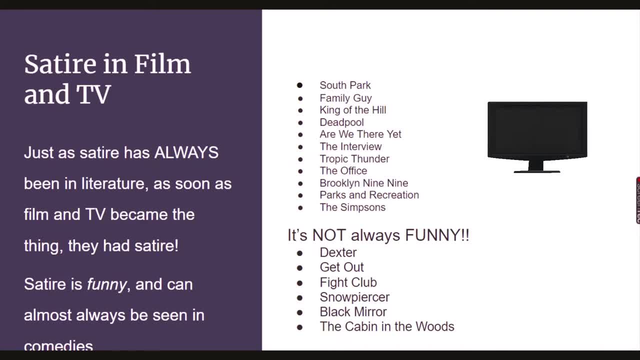 So, just as literature has always had some form of satire along with it, we've also seen satire in film and TV ever since film and TV became a thing. The reason is because satire is usually funny, And if it's not funny, it's ironic in a scary way. 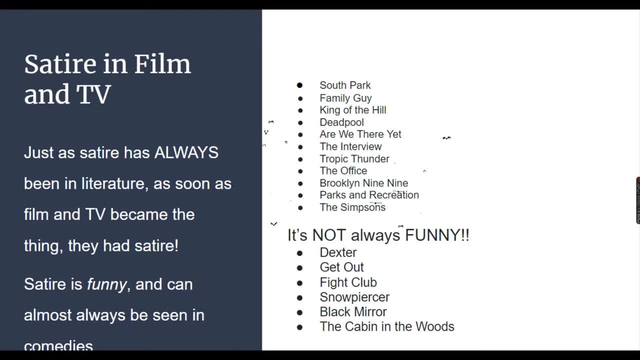 So it makes a real punch for people to think about. Just because satire can be funny doesn't mean it's always funny. A lot of TV shows that we have now are satires, but they're not funny at all: Dexter Get Out, Fight Club, Snowpiercer, Black Mirror and The Cabinet. 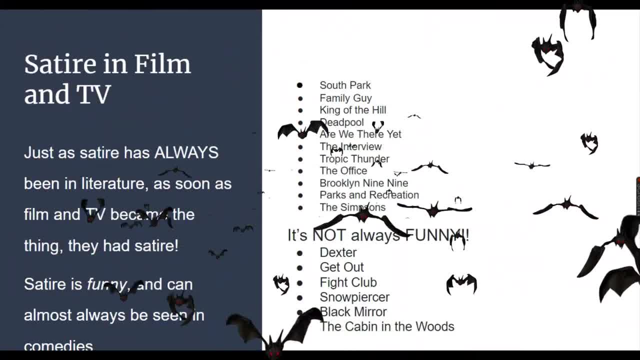 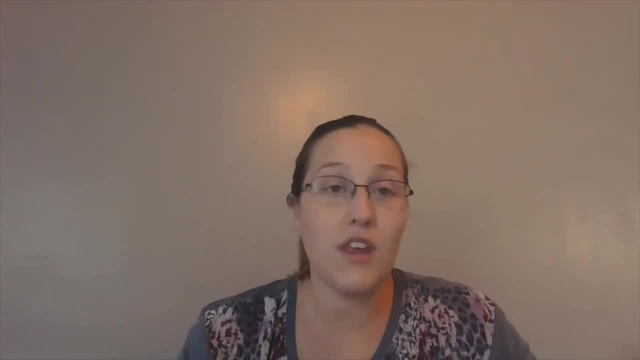 And The Cabin in the Woods are all examples of satire in film. that's not really funny, but definitely criticizing something going on in our world at the time that the film is taking place. The thing that you want to think about when it comes to satire is: why do we care? 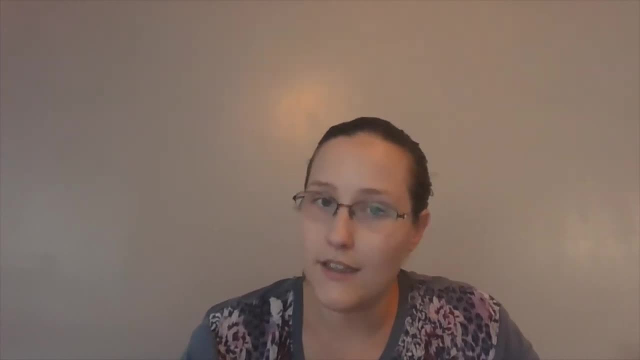 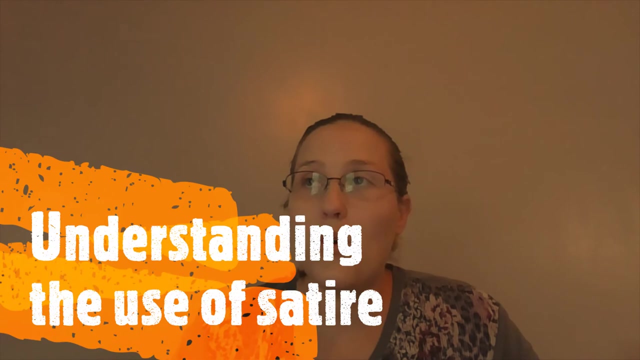 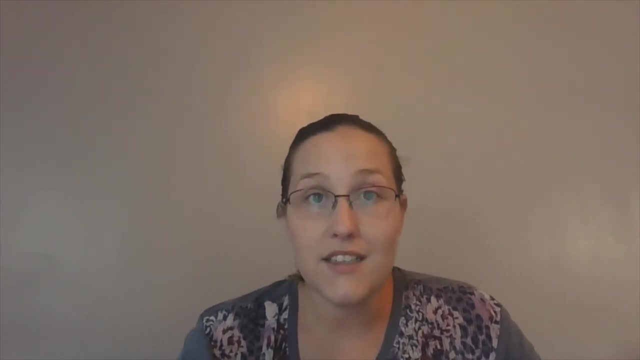 What's the point? As a student and as a person in society, it's important to understand what the use of satire is. So when people put satire in a story or when they put it in a movie, they're actually trying to get the audience- the readers or the people- watching. 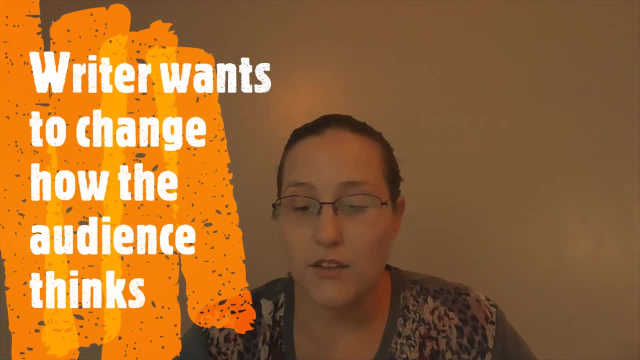 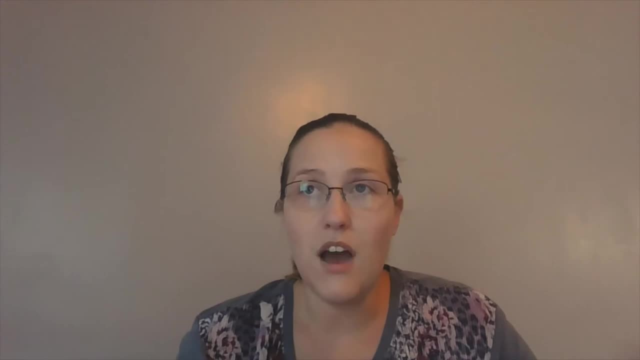 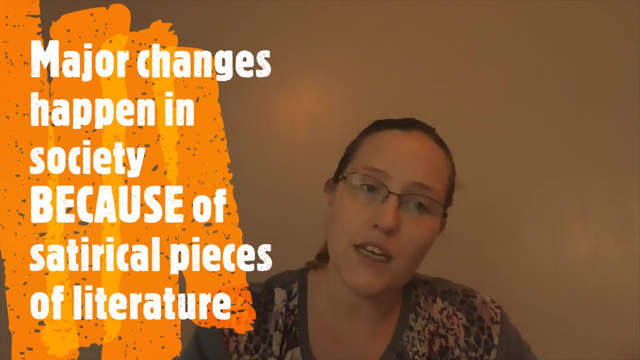 to change their way of thinking. They're trying to create a catalyst that will allow the audience or society to understand an issue and to decide to make a change. So what's really interesting is if you go back in history and you look at the authors that are writing the satire. 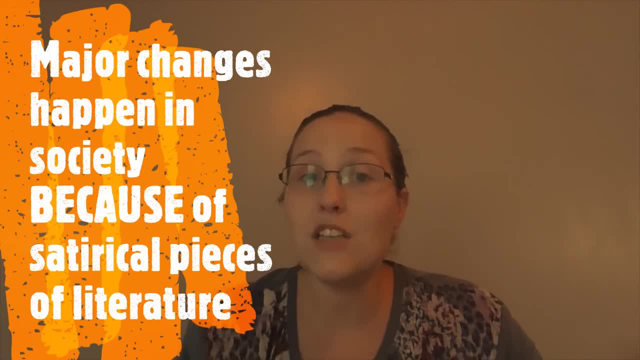 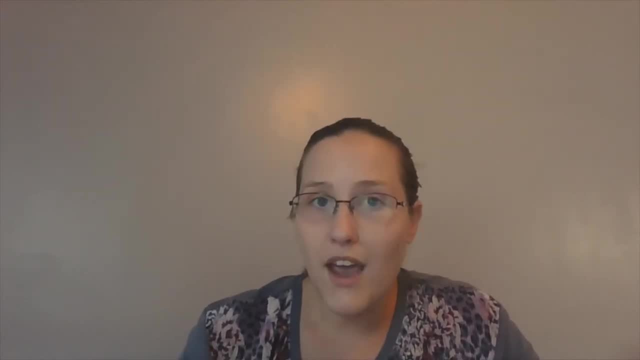 it's not very long after that you start to see historical changes in society. You start to see people realize that slavery is not okay, But the texts written about it would have come before. And then they became popular and those things made people think. 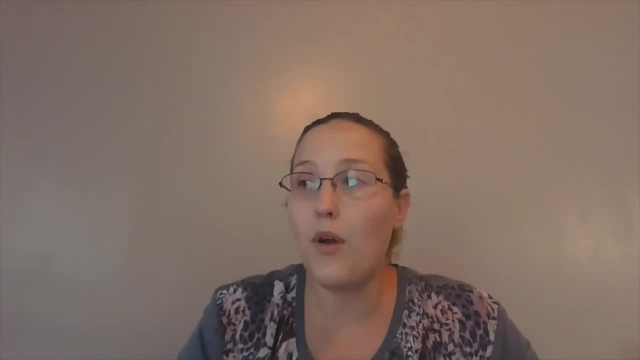 and it made society question itself and it brought about a bunch of changes. Now, a lot of times, society can make these changes on its own, but it is really interesting to see the things that are written right before major movements happen, because, you will see, satire comes first. 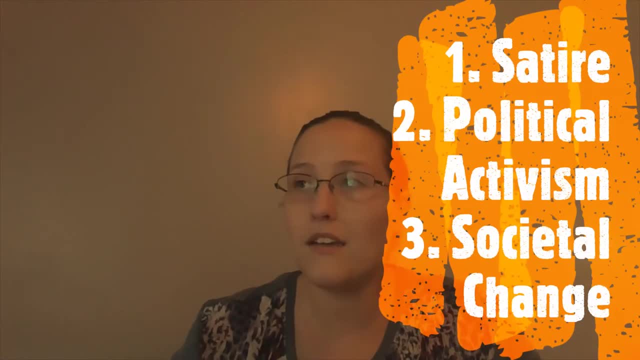 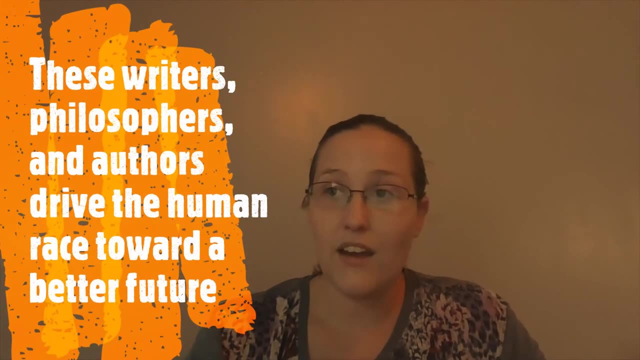 then comes political activism and then comes a change in society. So, if you're thinking about it, these writers, authors and philosophers are the ones that are driving our society, or the human race, in the trajectory that we are going, And it's really fun to connect history to literature like that. 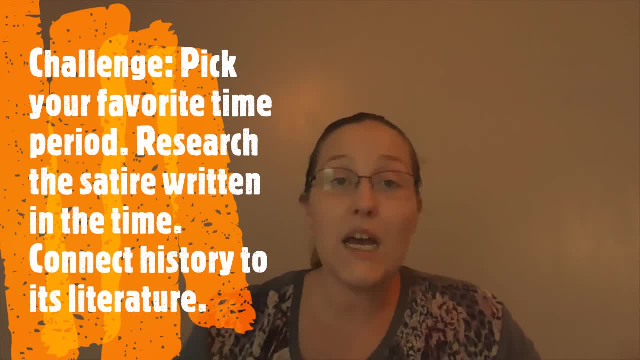 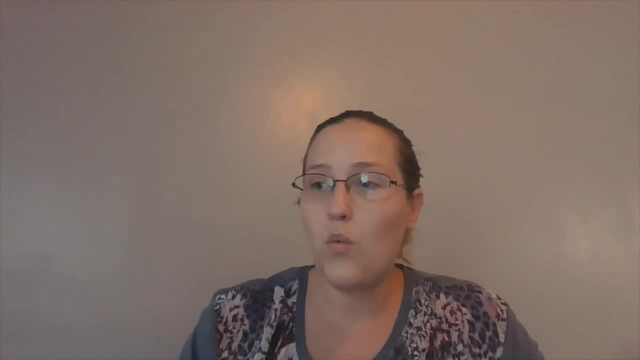 So I give you guys a challenge: Pick any time period that you really enjoy and go back and research the satire that was written at that time. Find out: was the writer successful in pointing out things that people had issues with? Was there a change or a shift in society shortly after the text was written? 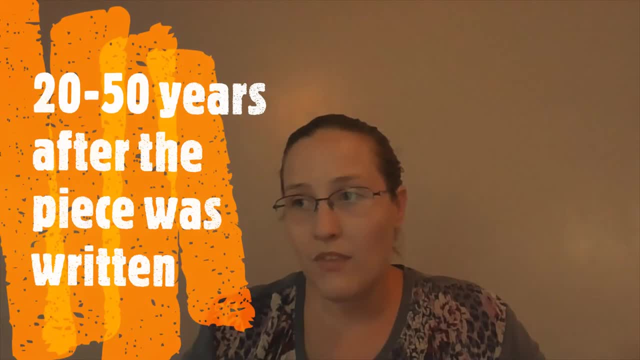 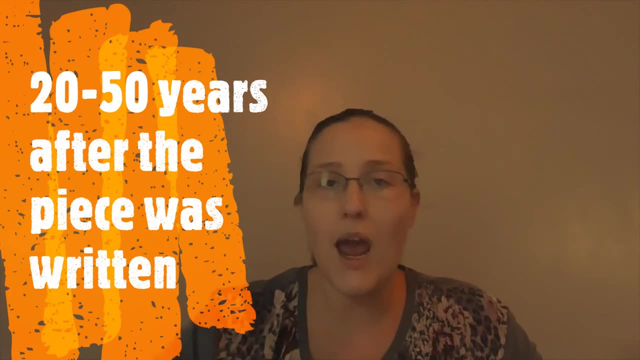 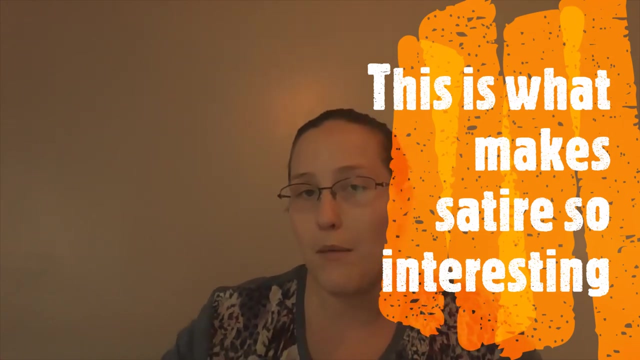 Now, when I say shortly after, I usually mean about 50,, 20 to 50 years from publication, when people are talking about an issue and actual real change in society. But obviously our society is not what it used to be. Things are happening that make people change. 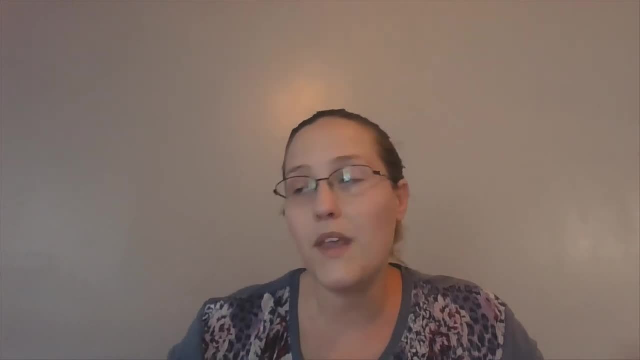 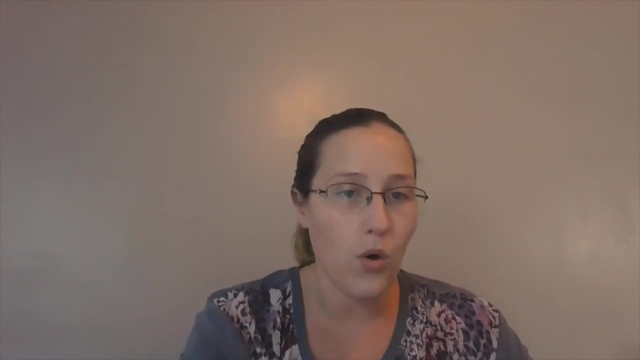 that make people question the status quo and what is happening. And that is why satire is so interesting, especially when you go back and look at it with history And you can see the shifts and the changes that people as a whole, that society, has made. 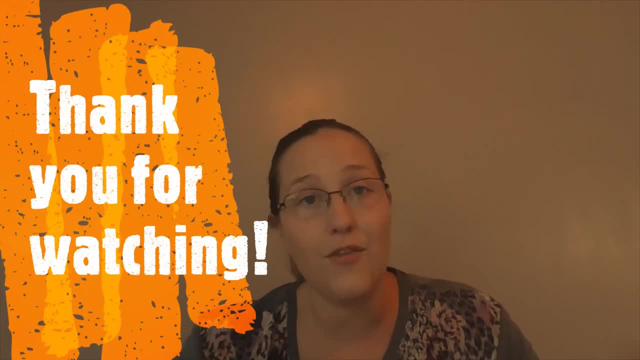 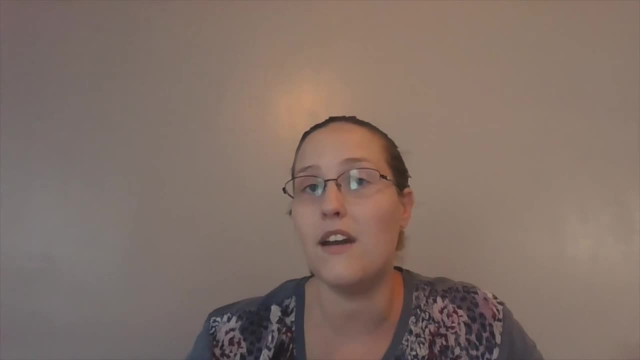 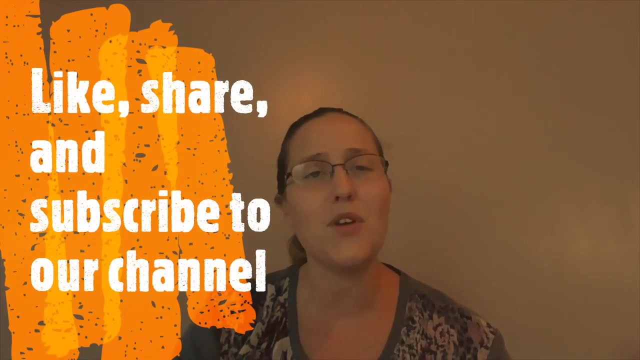 I hope you guys really enjoyed this satire video And I hope that you're able to think a little bit more about the importance of literature and even film in our society. Check us out next week. We'll have some more videos coming soon And I hope you guys like share and subscribe to our channel. Bye-bye.